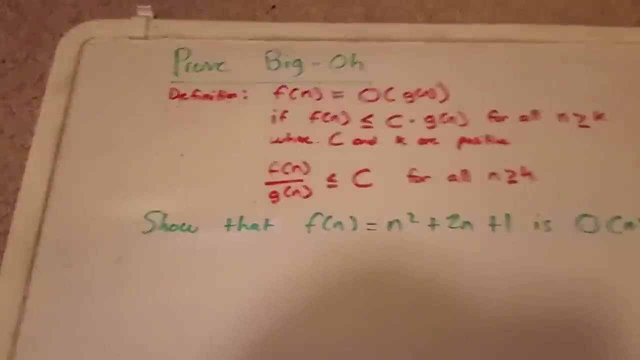 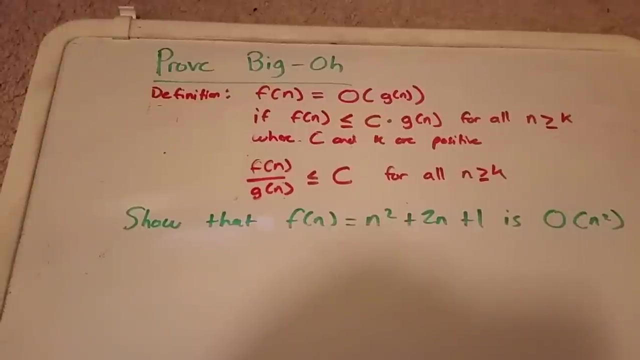 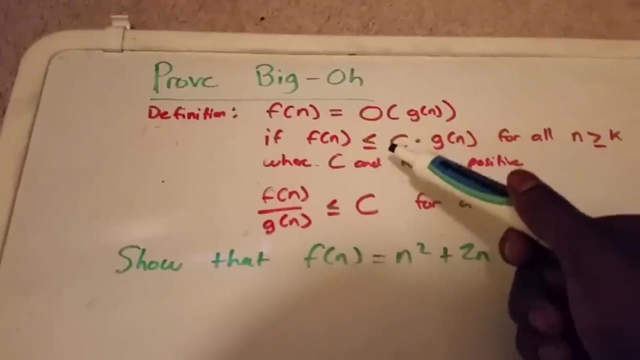 Hello YouTube. this is a Big O Proof. So before we even start the proof, we have to understand the definition of what it means for a function to belong to Big O. So here I wrote down a definition You have: f of n belongs to O, g of n if f of n is less than or equal to some. 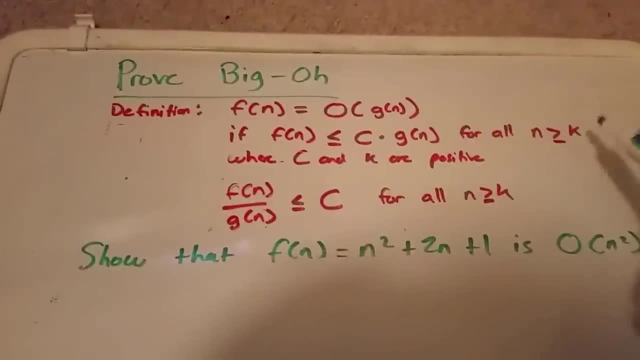 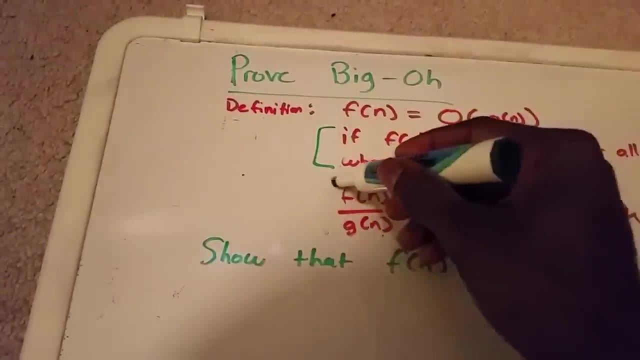 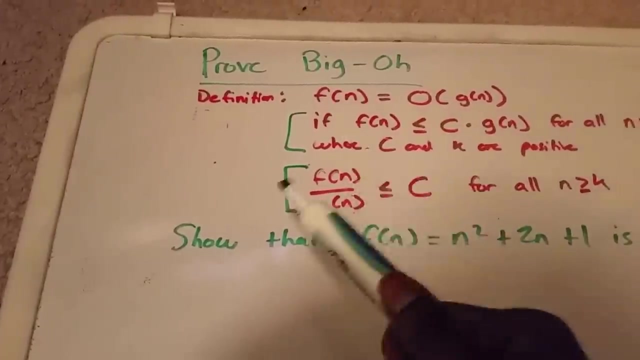 constant times, g of n for all n greater than or equal to some constant k, where c and k are positive constants. We can rewrite this equation here like this, such that now f of n belongs to Big O, g of n if f of n divided by g of n is less than or equal to some constant. 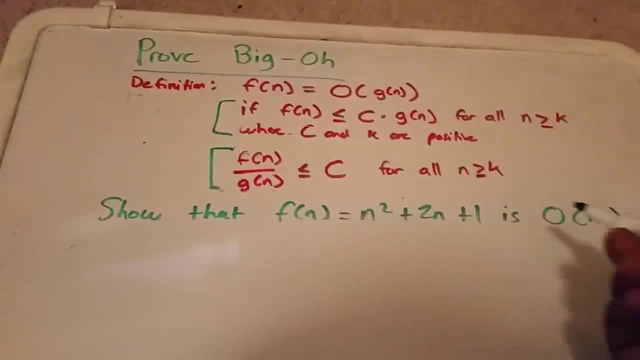 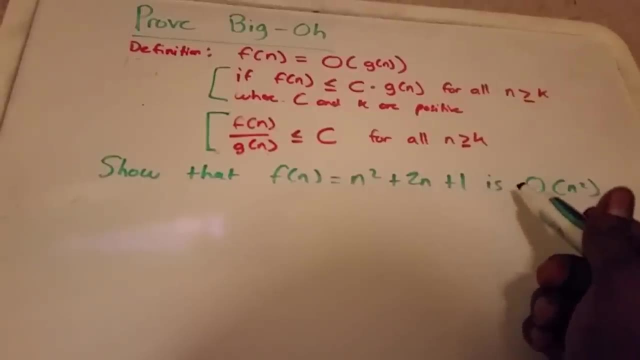 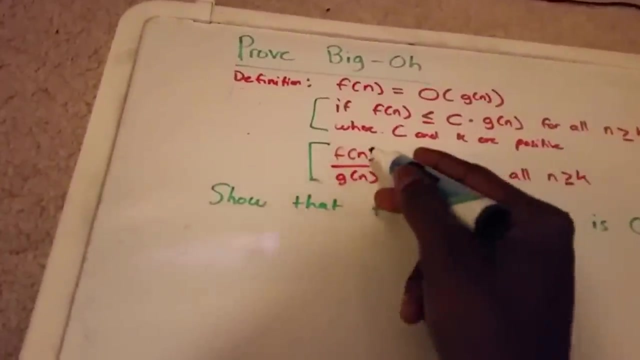 for all n greater than or equal to k. So here we have f of n equals n squared plus 2n plus 1.. We want to prove that it is a constant Big O of n squared or that it belongs to Big O of n squared. So rewriting this here: 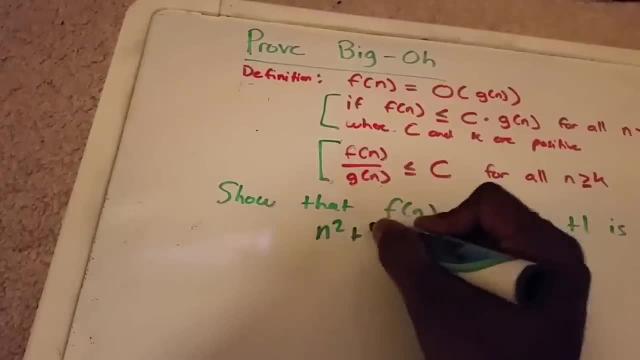 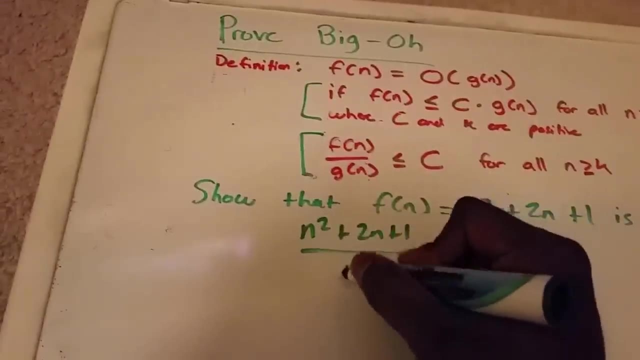 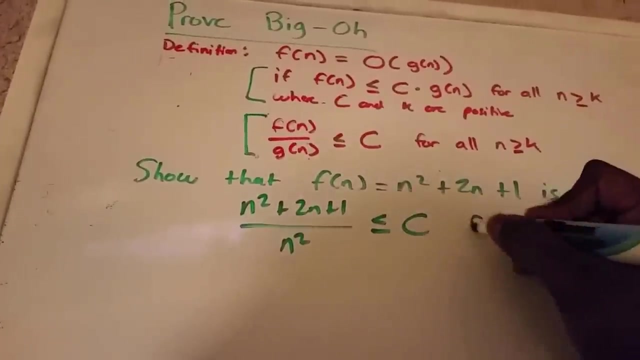 with what we have, we get n squared plus 2n plus 1. divided by our g of n is n squared And we want to prove that it is less than or equal to some constant for all n greater than or equal to k. 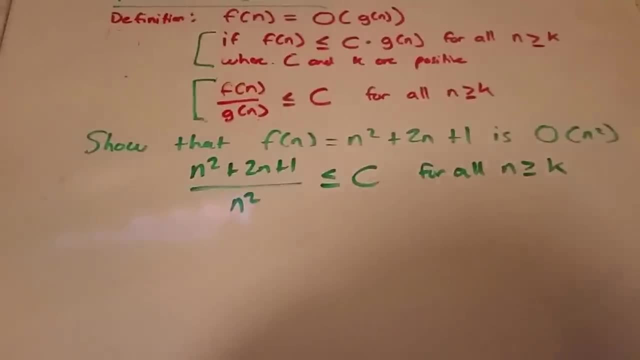 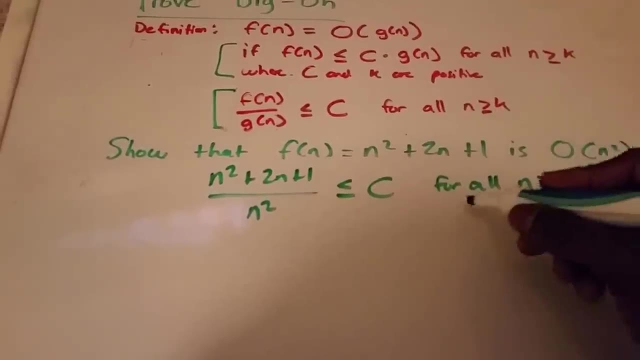 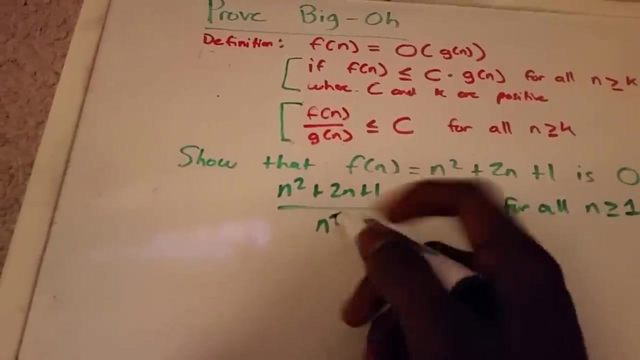 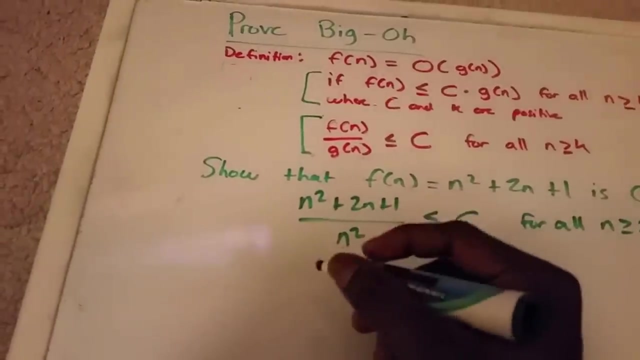 So let's choose k to equal 1.. So now we can write this here as for all n greater than or equal to 1. And we want to find a function bigger than this one. So what we can do is we can replace everything that's not as big as this one. So we can replace everything. 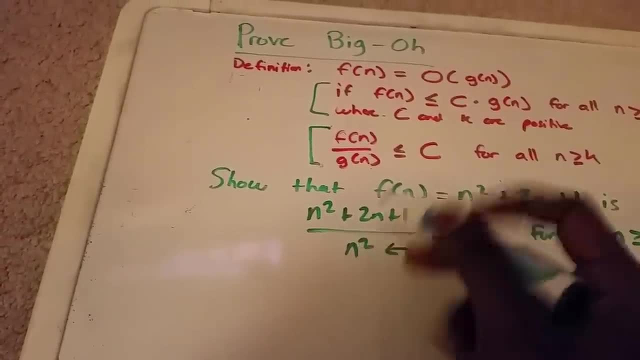 that's not as big as this one, So we can replace everything that's not as big as this one, So we can revalue to give us k. Now we can feel a constant, So we can feel our constant. Well, let's hommes, we can read this as: 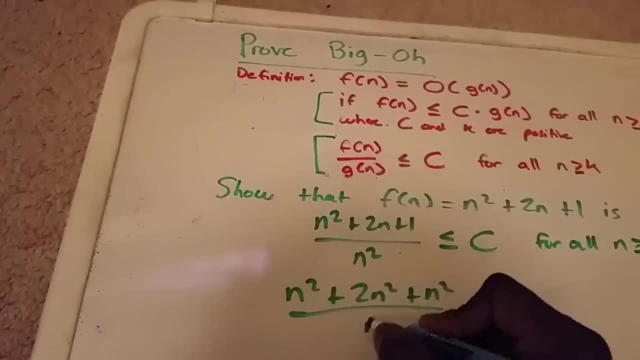 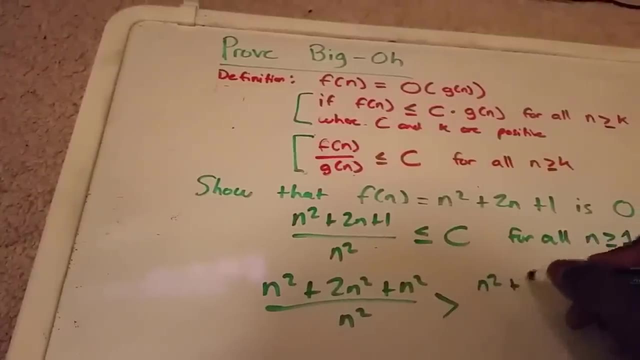 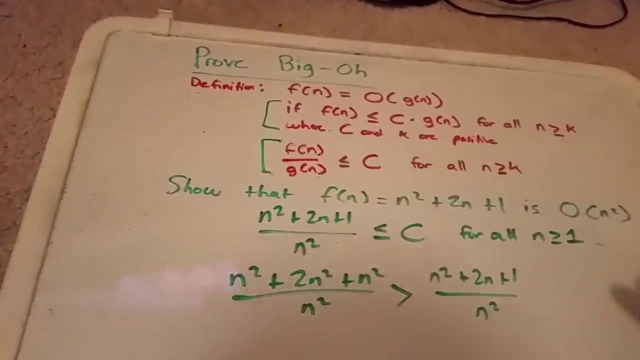 this constant n. Let's hopes that our constant is the right over n Great. All right, We got some potassium. There's only some potassium left. but we'll take that to give the variable n squared as what we're dividing by. We know that n squared plus 2n squared plus n squared all over n squared is greater than n squared plus 2n plus one over n squared. for all n greater than or equal to G over n greater than n squared greater than bn greater than or equal to g over all n greater than n squared. 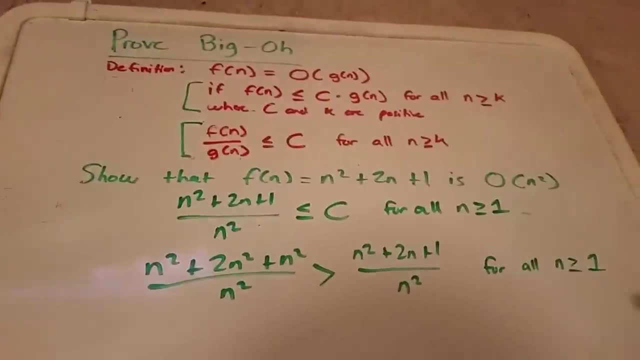 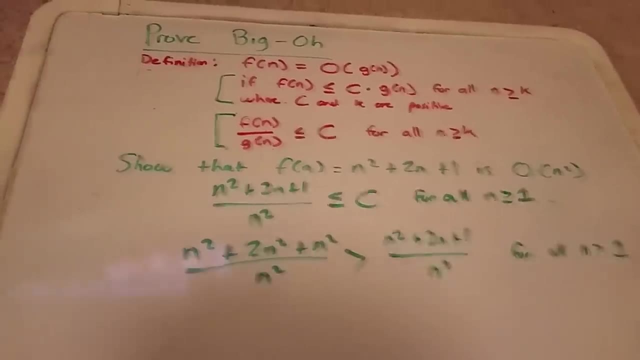 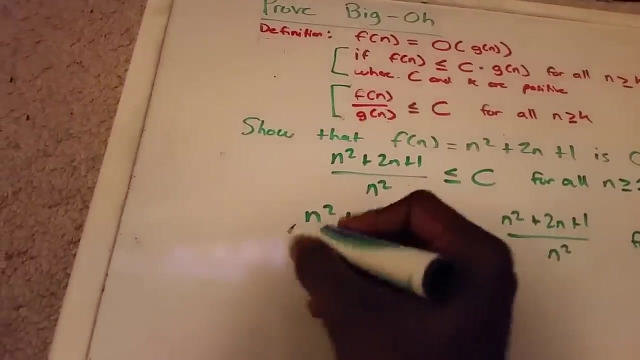 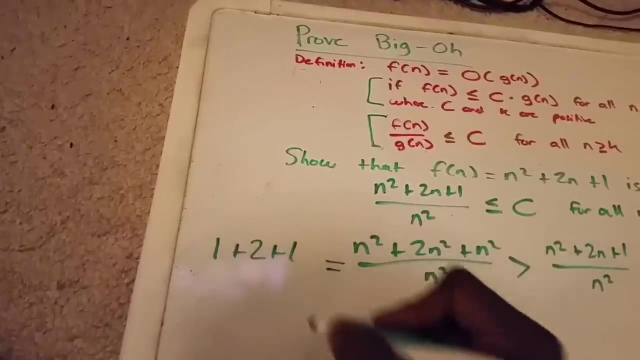 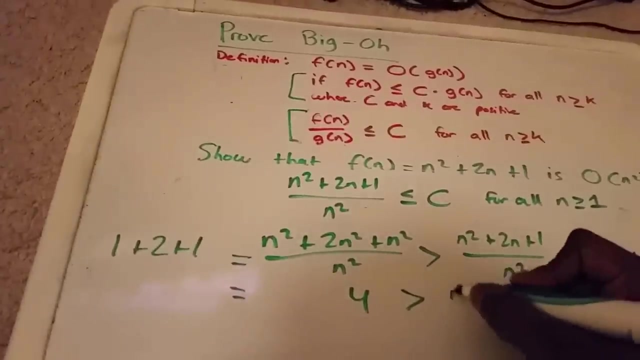 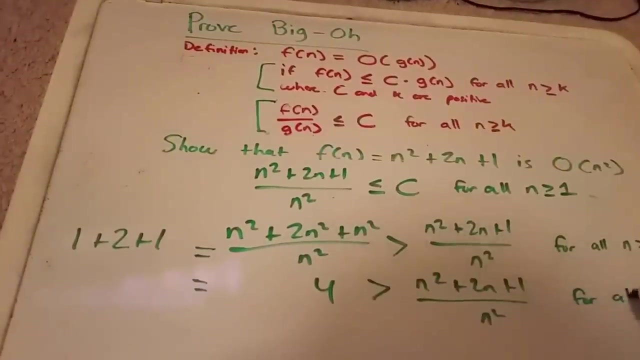 Greater than or equal to 1.. Well, actually, for all n greater than 1.. So what this means is this: equals 1 plus 2 plus 1.. So it equals 4.. So that means that 4 is less than I mean. 4 is greater than n squared plus 2n plus 1 over n squared for all n greater than 1.. 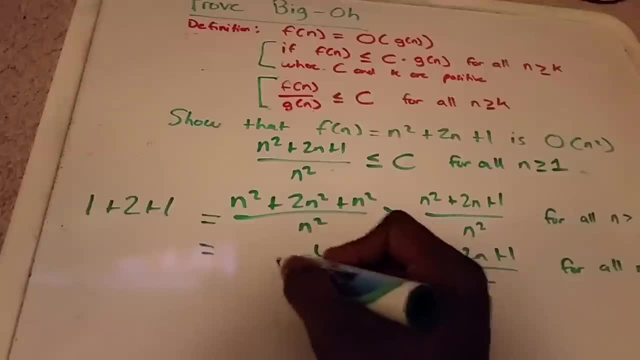 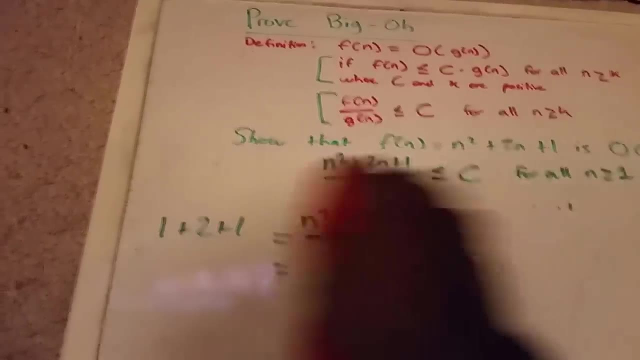 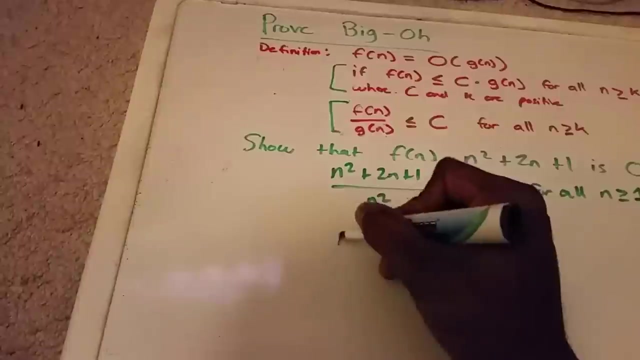 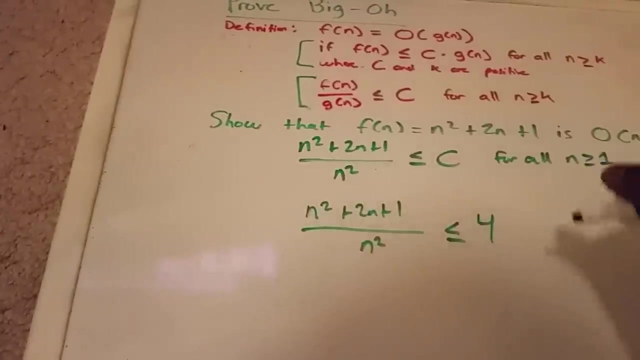 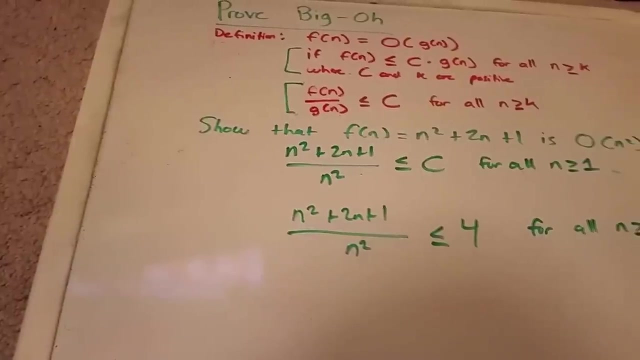 So let's choose our constant to be 4.. So now we're going to let c equal to 4,, such that n squared plus 2n plus 1 over n squared is less than or equal to 4.. For all n greater than or equal to 1.. 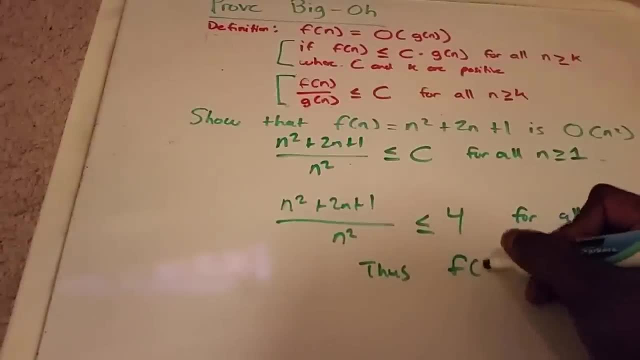 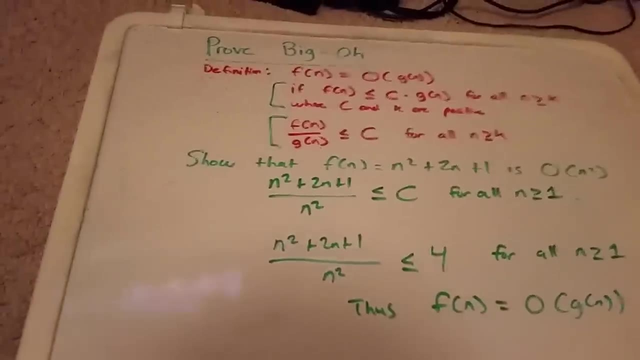 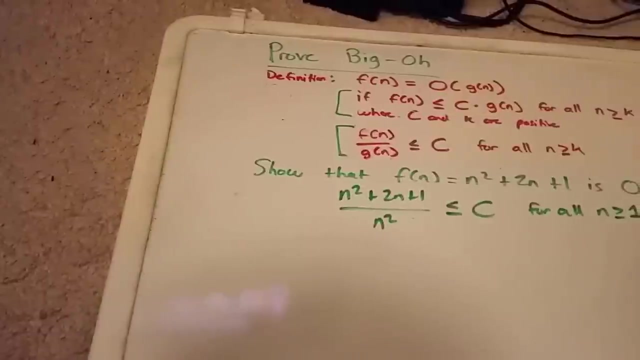 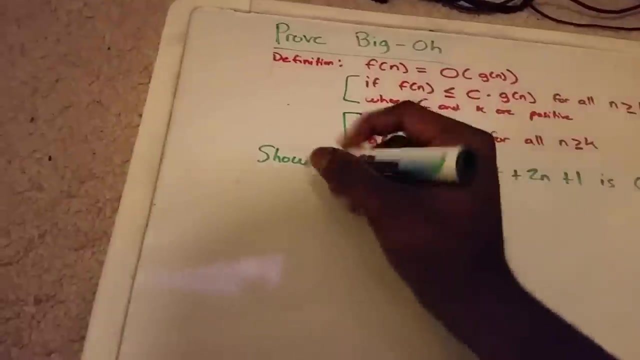 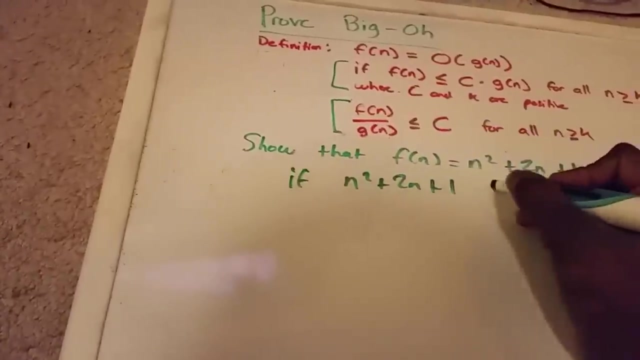 Thus f of n belongs to big O g of n. Alright, And another way to see this is for us to use the first definition. So if n squared plus 2n plus 1 is less than or equal to some constant, 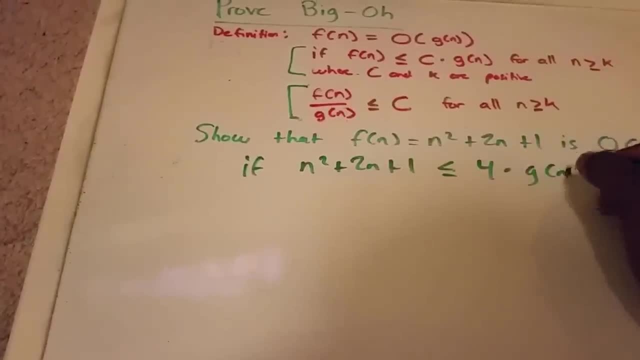 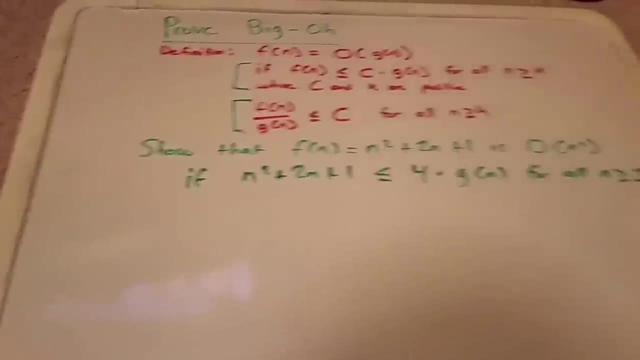 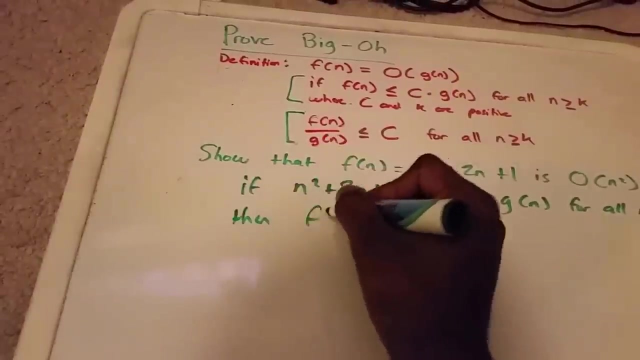 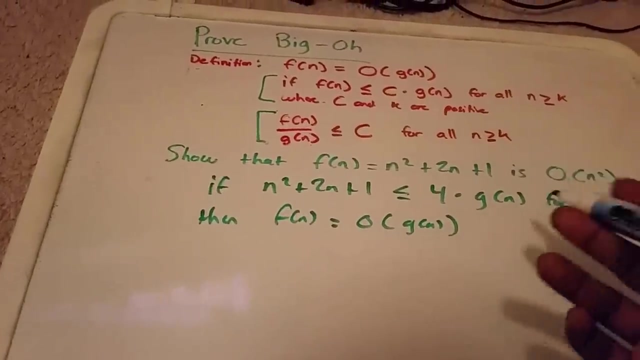 we said, our constant is 4 times g of n for all n greater than or equal to 1.. Then we know, f of n belongs to big O of g of n. Alright, Here our g of n is 4 times n squared. 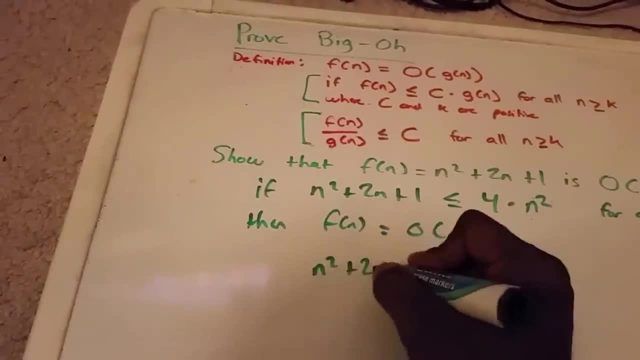 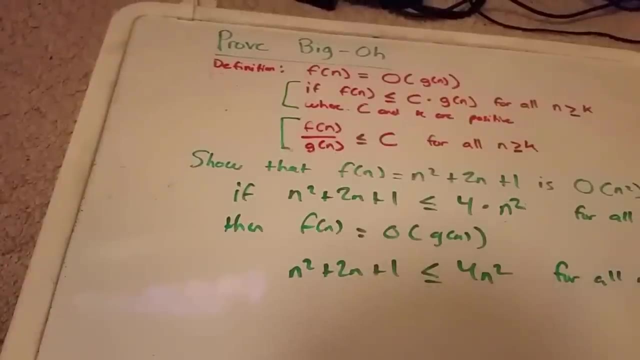 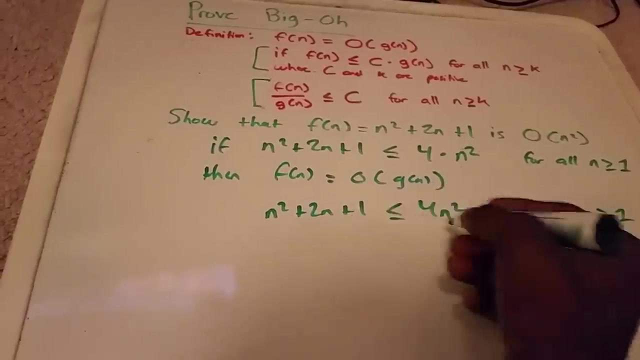 So let's prove this: Square plus 2n plus 1, that's is equal to 4 times n, squared for all n greater than and equal to 1.. So let's subtract from both sides So 2n plus 1. 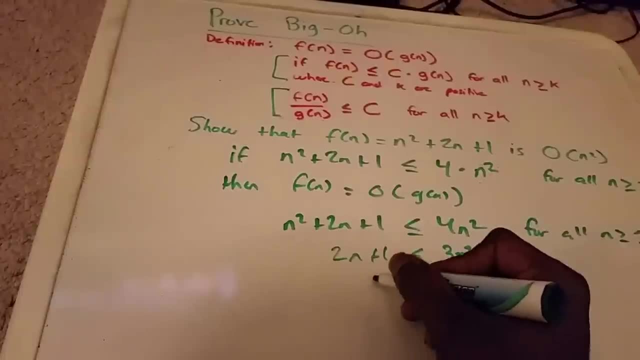 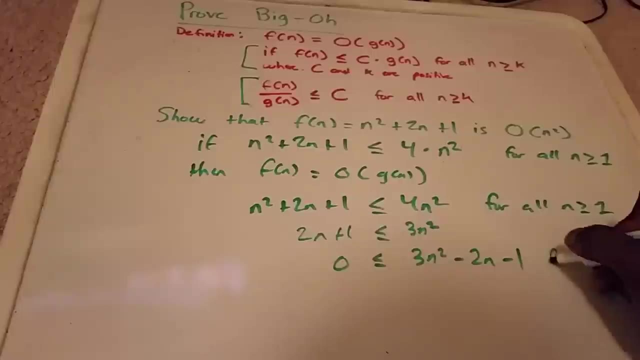 less than or equal to 3n squared. And we have, yes, And we have 0 less than or equal to 3n squared minus 2n, minus 1.. And we can't forget the for all n greater than or equal to 1.. 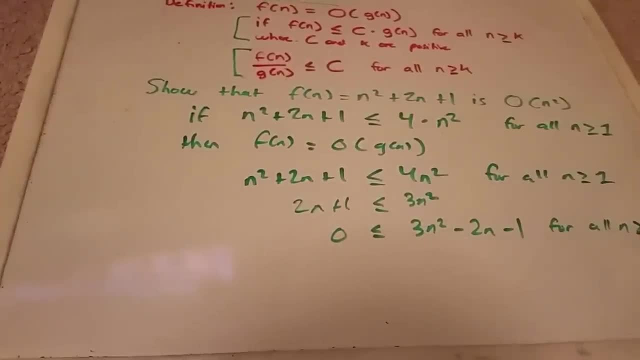 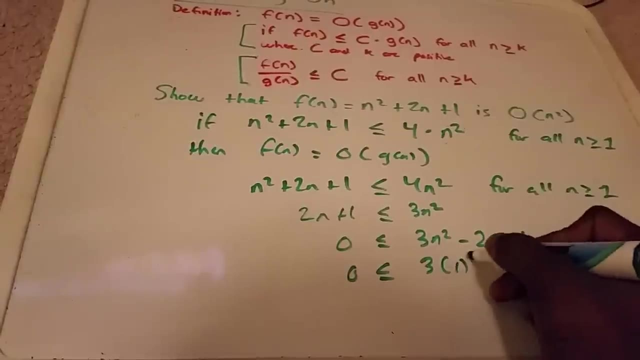 So the lowest value n can be here is 1.. So let's plug in 1 here: 0 less than or equal to 3 times 1 squared minus 2 times 1 minus 1.. And we can rewrite that: 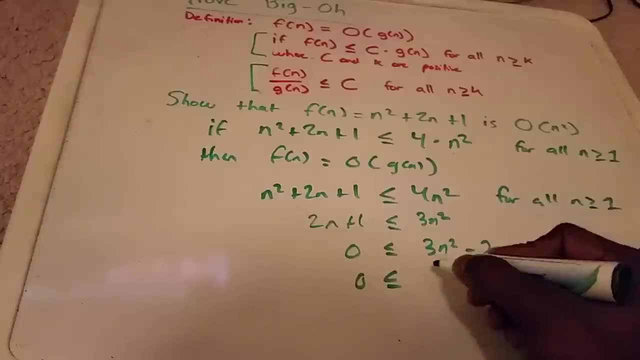 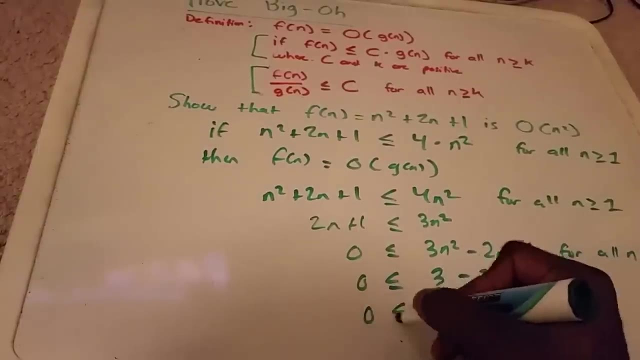 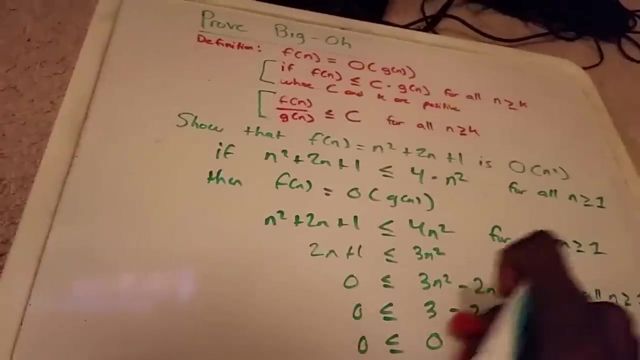 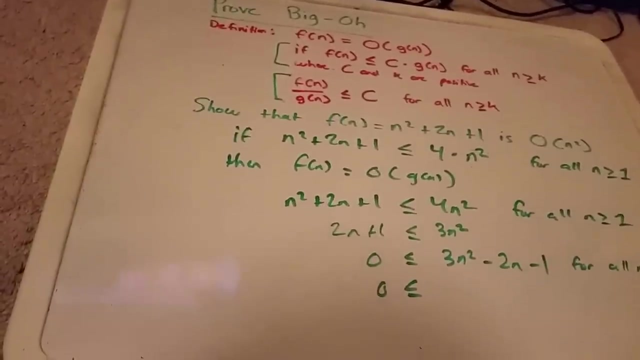 0 as 3 minus 2 minus 1.. So 0 less than or equal to 0.. Okay, So that is true. So let's try another value. Let's choose: n equals 2.. So now we get 3.. 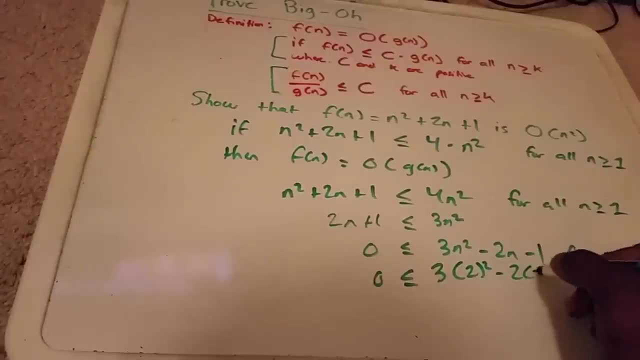 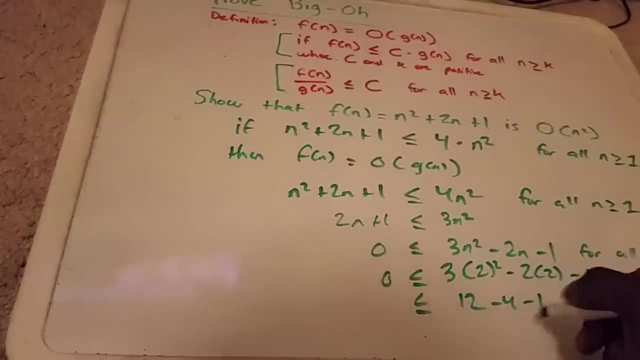 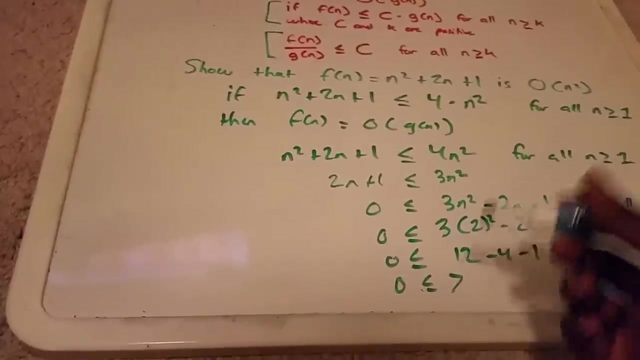 Times 2 squared minus 2, times 2 minus 1.. Less than or equal to 12 minus 4 minus 1.. So 0 less than or equal to 7.. And you can see that this continues for all n greater than or equal to 1.. 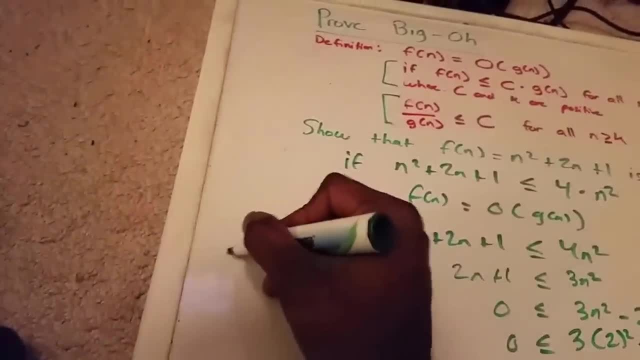 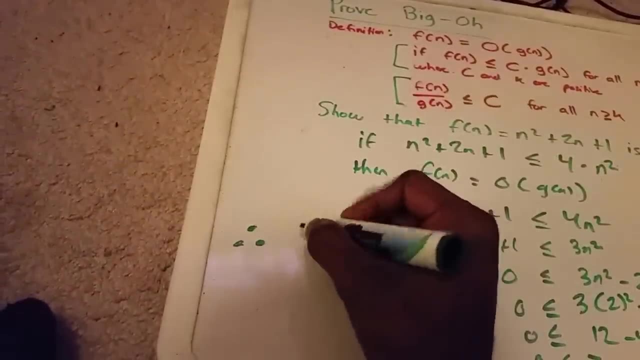 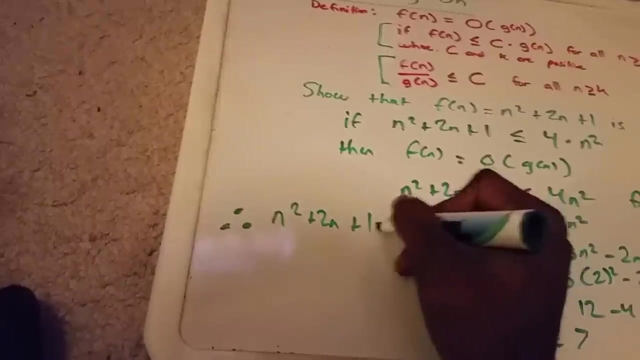 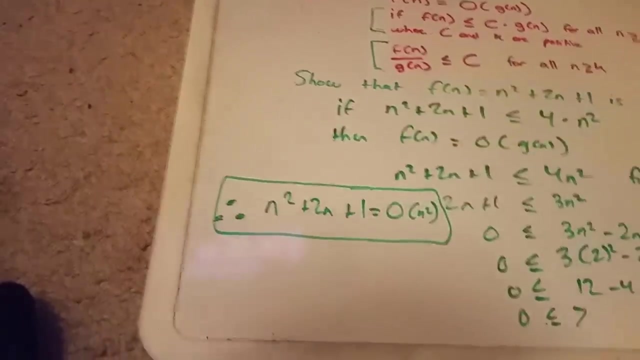 So therefore, Let's use that nice little three dots. Therefore, that's what the three dots mean: n squared plus 2n plus 1 equals big O of n squared. Alright, Thank you.